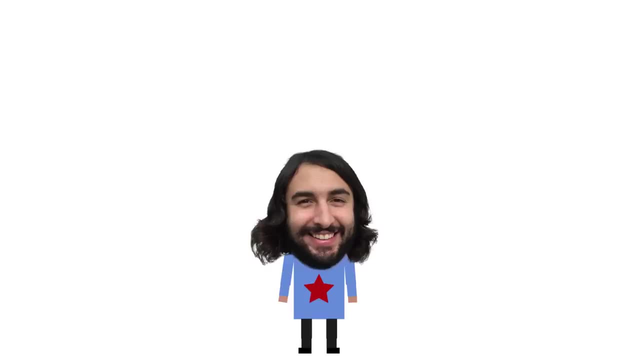 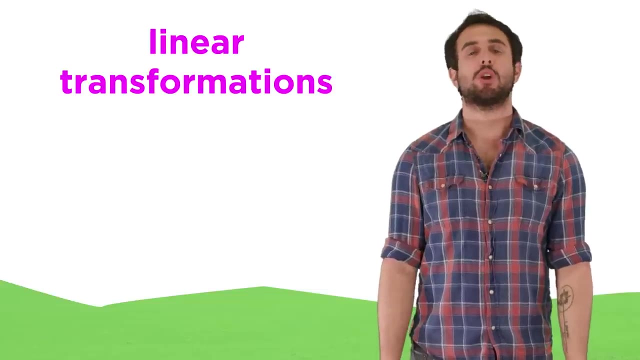 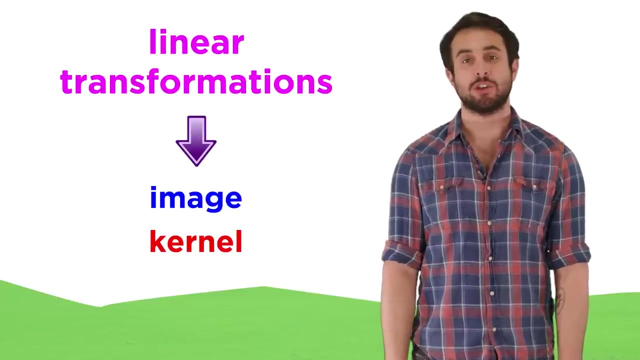 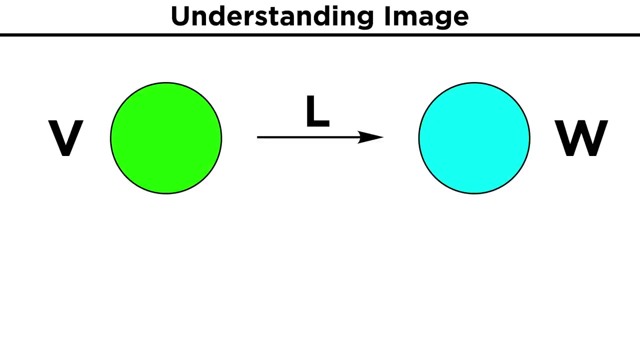 Professor Dave, again let's talk image and kernel. Now that we have learned about linear transformations, we have to discuss two related concepts, and these are called image and kernel. These are best defined by example, so let's take a look at one now. 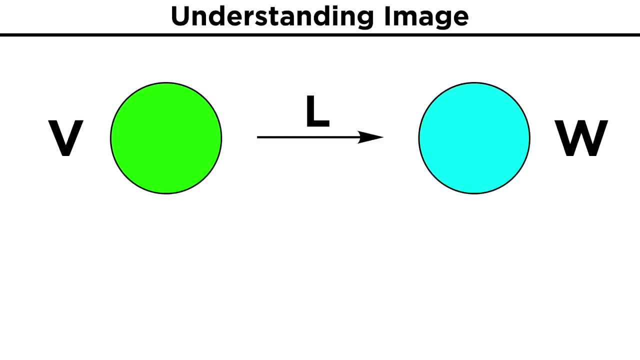 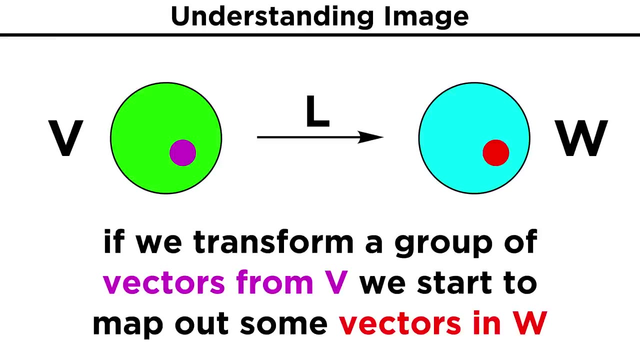 Say we have a linear transformation that maps from the vector space V to the vector space W. As we know, this will involve taking vectors from V and turning them into vectors in W. If we transform a group of vectors from V, we end up starting to map out several vectors. 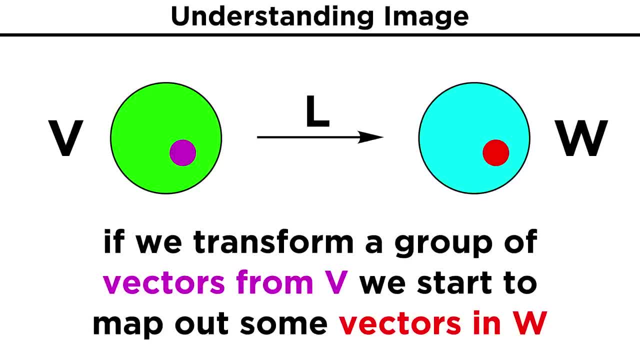 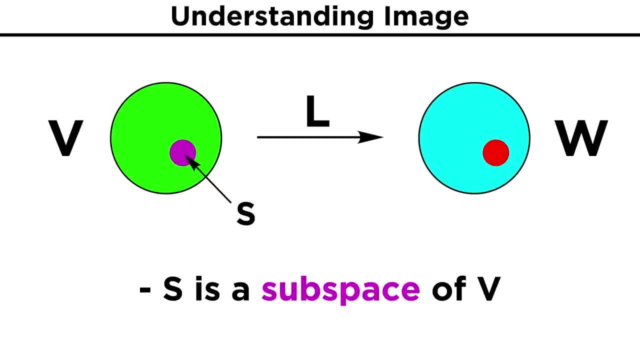 in W. This is the idea behind what we mean by image. If we take a subspace of V, let's call it S. this is a group of vectors from V that can then be transformed. The set of vectors that we can get from this transformation is what is known as the image. 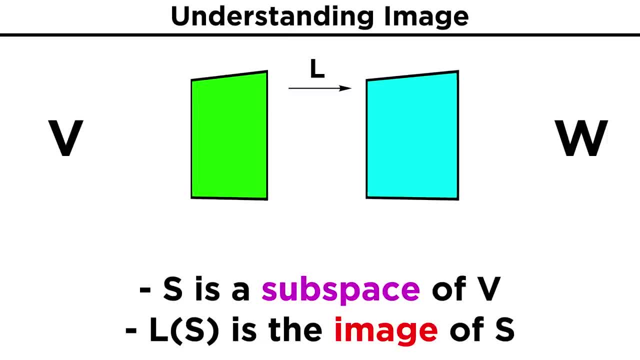 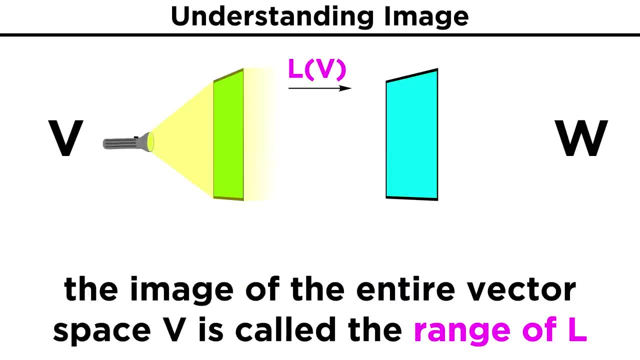 of S. One way to think of it is that it's as if we are shining a light on a part of the vector space V and seeing how much of W gets lit up. The area of W that gets lit up is our image. 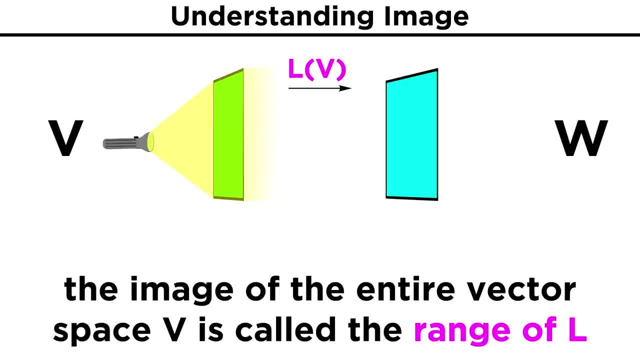 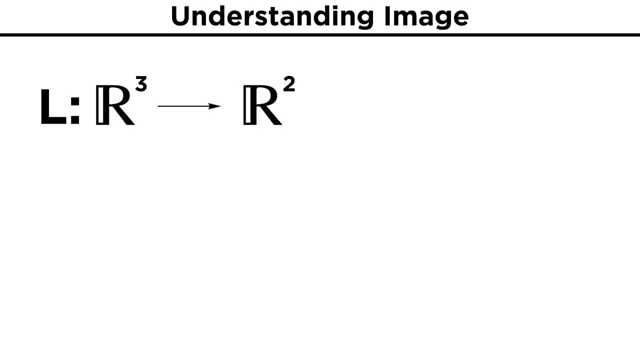 The image of the entire vector space. V denoted this way, has a special name. It is called the range of L. For example, consider the linear transformation that maps R3 to R2, given by L of V equals V1, V2 minus V3, for any vector in R3. 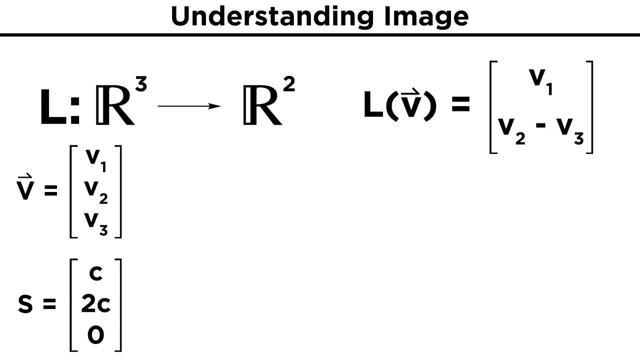 For this example. let's say our subspace of V is given by the vectors of length three, where the second element is two times the first element and the third element is zero. Written out, this is the set of vectors of the vector space V. This is the set of vectors of the vector space V. denoted this way has a special name. 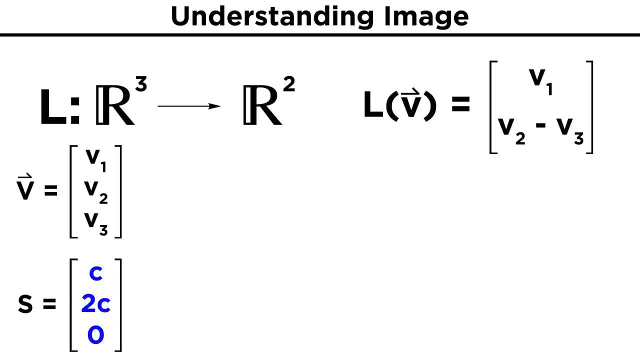 It is called the range of L. The image of the form C two, C zero, where C is any scalar. Let's plug this form into our linear transformation and see what we get. Our transformation says to plug the first element into the top row, so C, then plug. 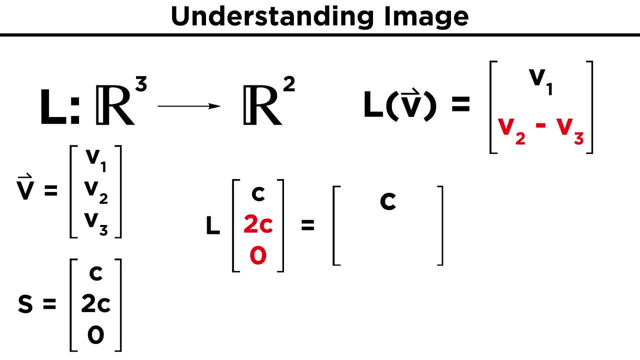 the difference of the second and third element into the bottom row. so two C minus zero, We end up getting an image of the form C two C. The image of our subspace is the set of vectors of length two, where the second element is twice the first. 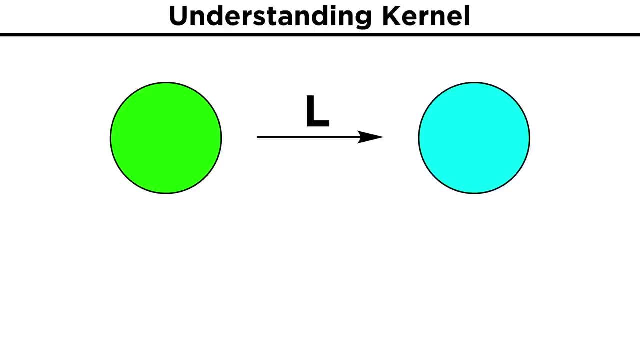 Now let's move on to kernel. Keeping in mind the fact that our linear transformation maps from V to W, the kernel of L, denoted as shown, is the set of vectors in V that, when transformed, become the zero vector in W. To keep zero vectors distinct, we will write the zero vector from V as zero zero. 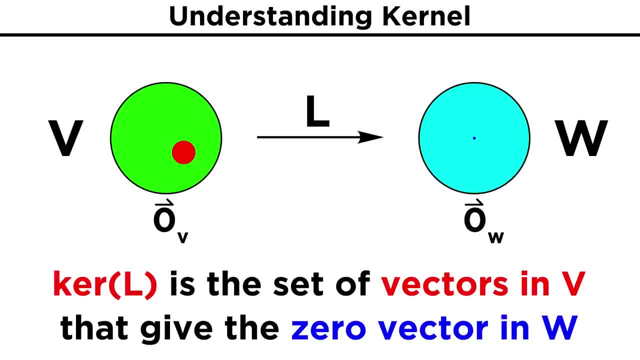 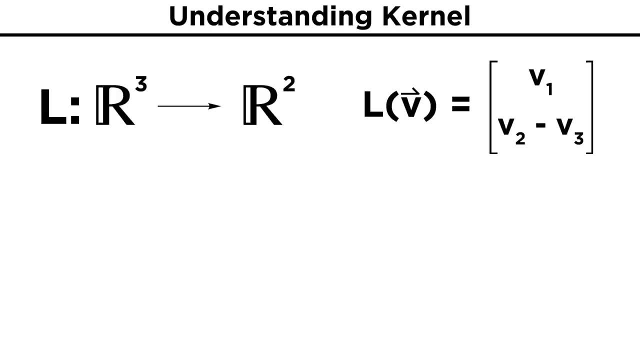 zero sub V and the zero vector from W as zero sub W. Let's take our linear transformation from earlier for an example. We have the mapping from R3 to R2, given by L of V equals V1, V2 minus V3.. 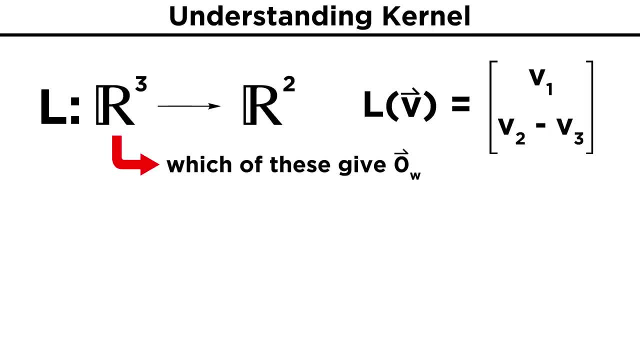 To find the kernel. we want to find which vectors in R3 give zero W under this transformation. This just ends up boiling down to solving the equation L of V minus V2.. We can find the vector in R3, and we can find the vector in R3. 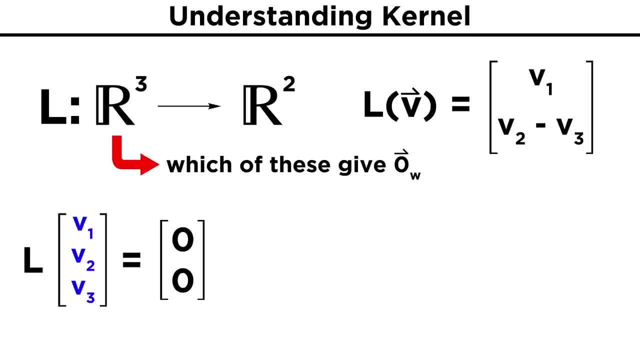 We can find the vector in R3.. Let'sception of L of V represents: L of V equals zero W for possible values of V1,, V2, and V3.. In this case that will be as follows: V1, V2 minus V3 equals zero zero. 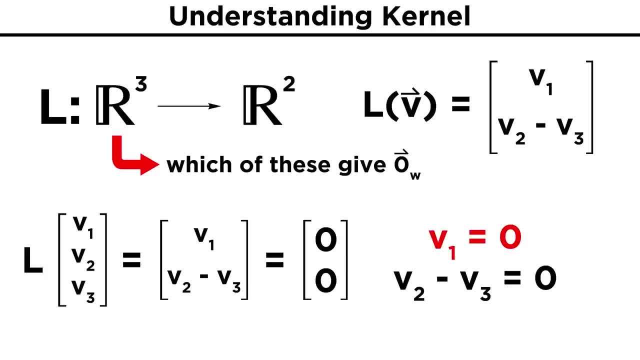 This reduces to a simple pair of equations: V1 equals zero and V2, minus V3, equals zero. Solving these gives us V1 equals zero and V2 equals V3.. This means that any vector from R3 of the same vector and the vector from the second. 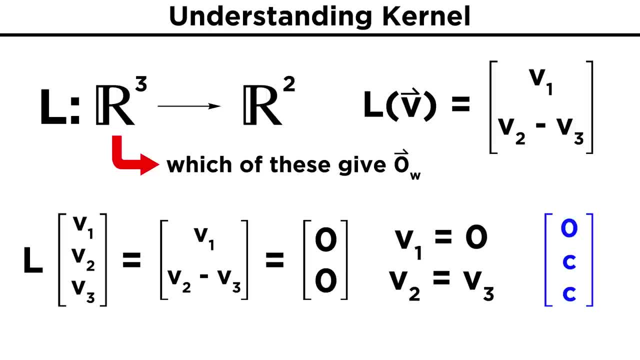 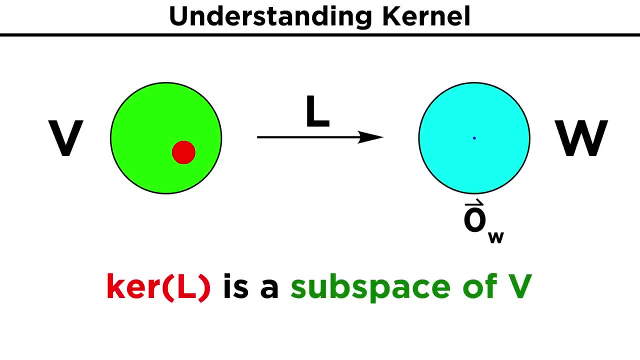 the form where the first element is zero and the second and third are equal to one another will give the zero vector in W when transformed. The set of vectors of this form is our kernel. Before we move on, it's worth noting that the kernel of L is a subspace of V and for any